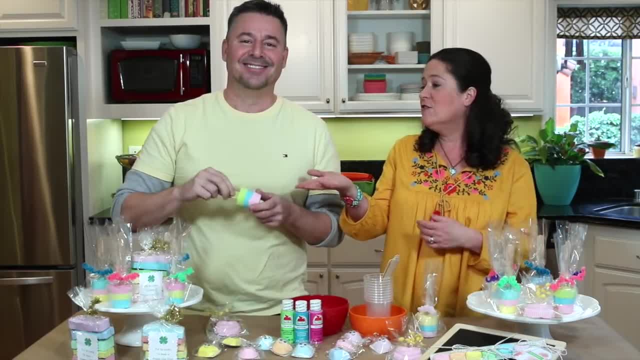 Perfect for the sidewalk, not for the bed? No, I don't think so. Hey, those wax cups though. that's a really cool mold. Oh, they work And so inexpensive- Perfect. Now there's lots of different things that you can use to mold your chalk, Some household. 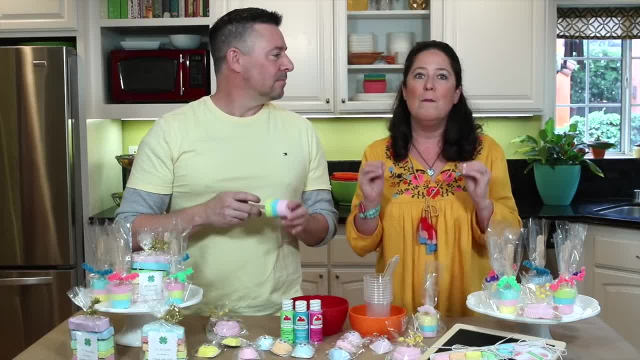 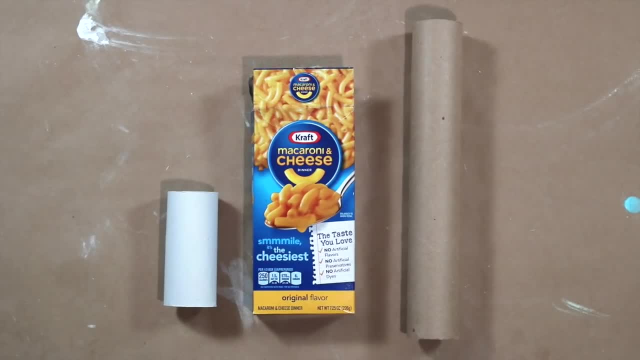 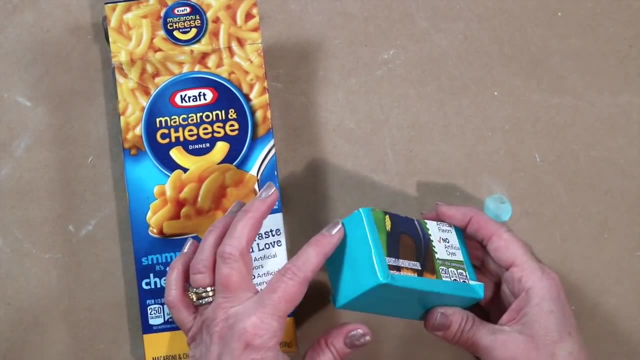 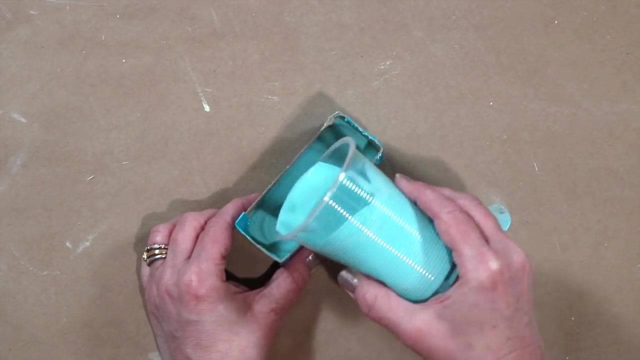 Recyclables. You can use recycle tubes and boxes to create chunky chalks. To create chalk bricks, I like to use macaroni and cheese boxes. Just cut the bottom off and add a little tape to seal the edges, Fill and allow to dry overnight. 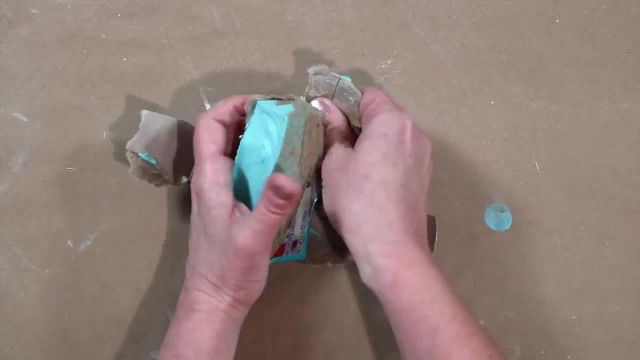 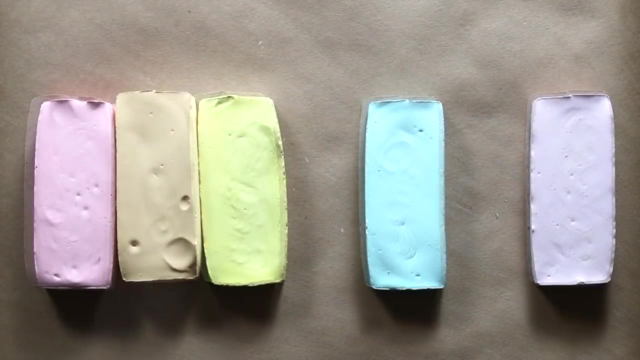 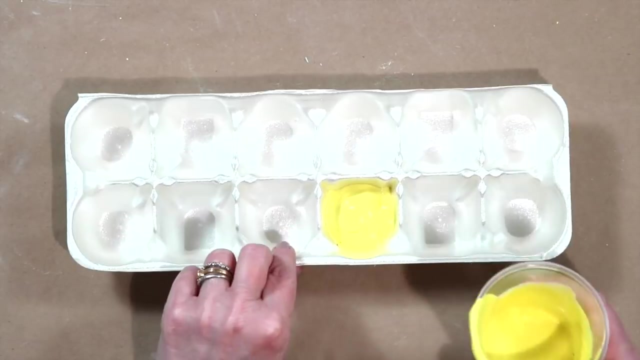 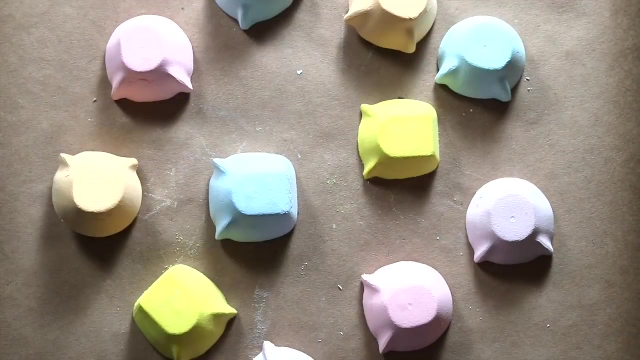 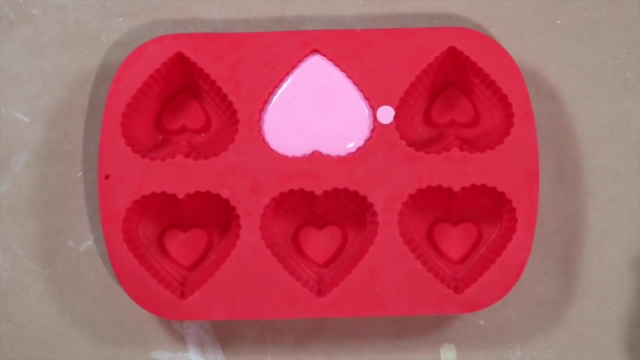 Peel away the box, Put it in the refrigerator. Egg cartons can be used to create cute chalk nuggets. We're going to be turning ours into animals. Large silicone baking dishes can be used to create large shaped chalks. Silicone candy molds are perfect for petite chalks. 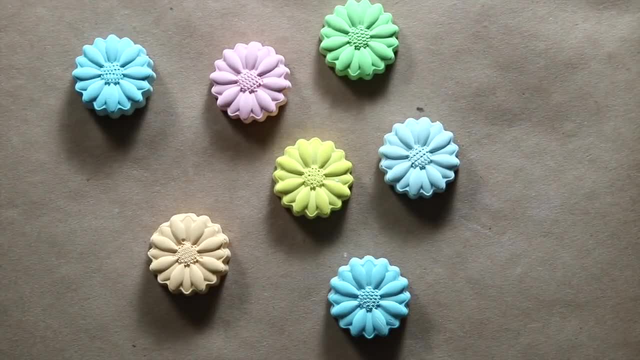 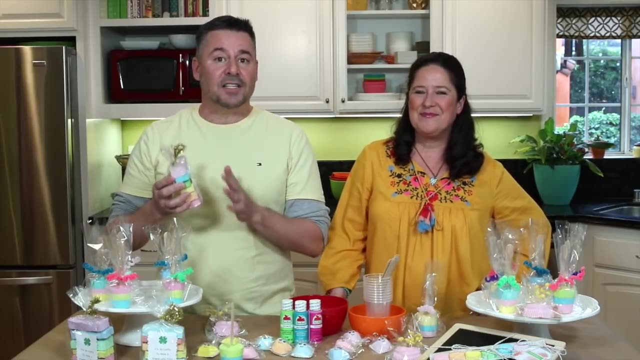 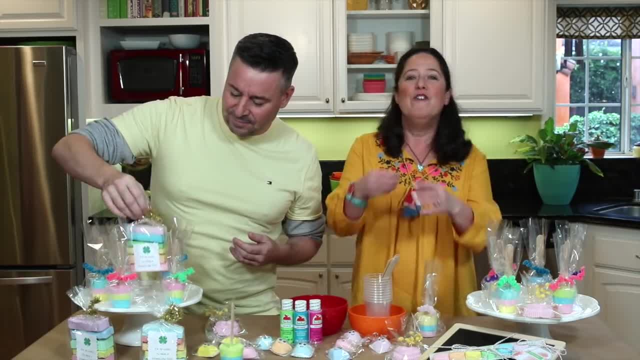 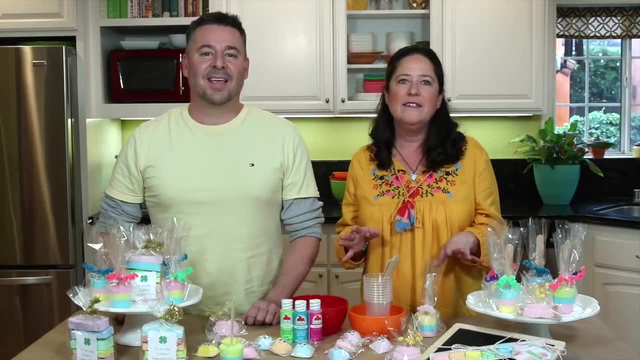 different colors using the apple barrel paint, And the colors are so pretty, Beautiful, Pretty For me. I'm always needing these little gifts for the girls to give to their friends or their classmates, so I really like the idea of them working with me to create the chalks. 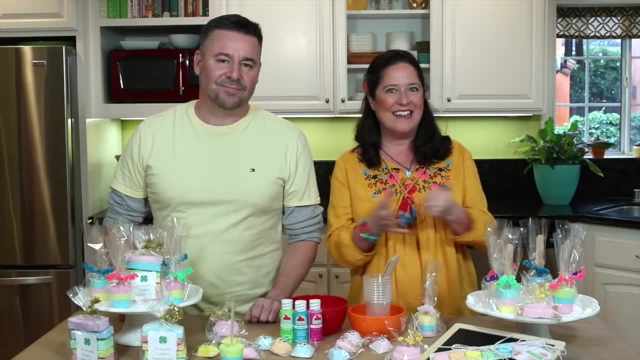 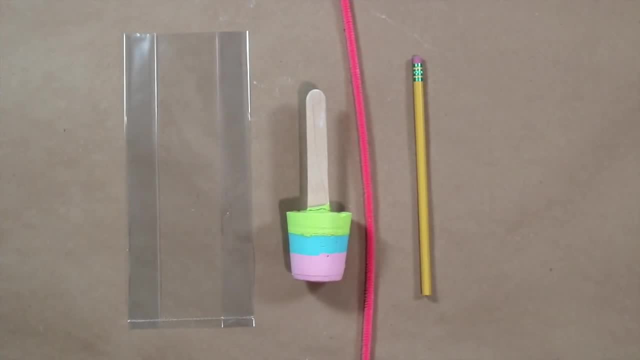 and then giving them as gifts. Yeah, Handmade gifts, It's always the best, Exactly The best, The best. Next, we're going to show you how to wrap all these up using cello bags. Turn the chalk pops into party favors.